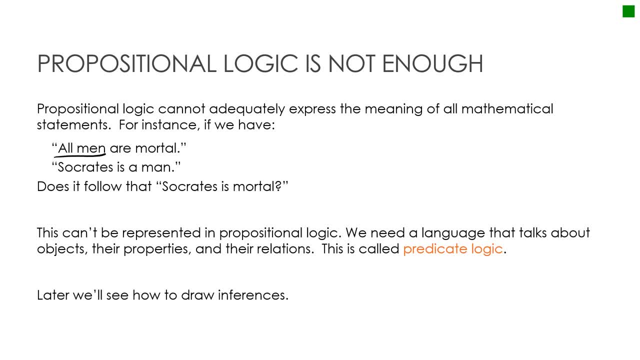 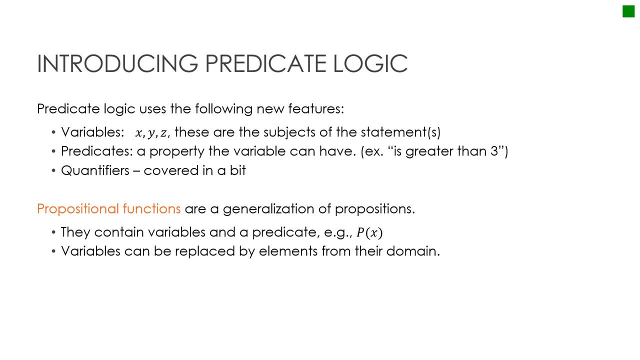 say all men, or what if it said some men, etc. So we can't represent that in propositional logic. We have to use something called predicate logic. Predicate logic uses variables, and variables are the subjects of the statement or statements. 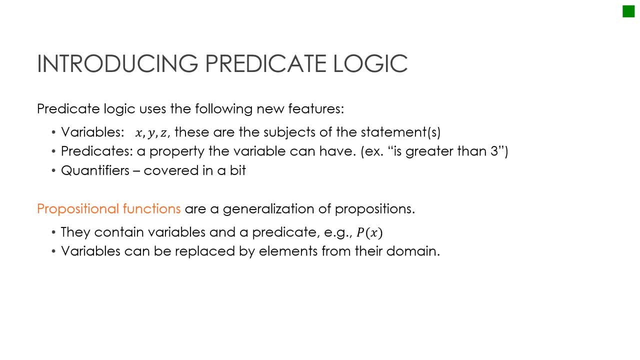 We use predicates, which is a property that a variable can have, like x is greater than 3, x would be our variable. is greater than 3 would be our predicate, and we'll talk about quantifiers in a little bit. So a propositional function is: 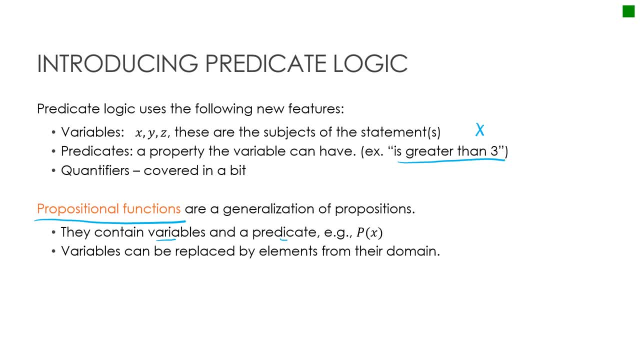 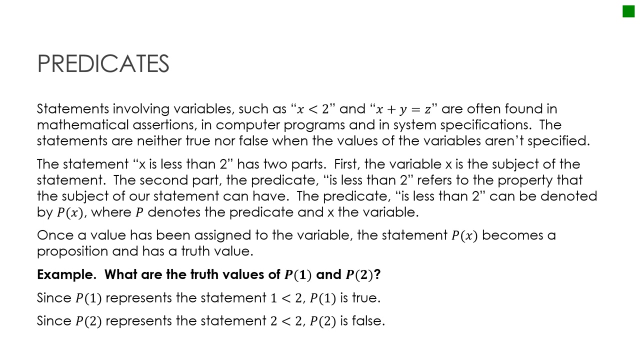 contains the variable and contains the predicate, And we use sort of a function notation for that because they are propositional functions. So p of x and again, just like in a propositional function, I can replace x with an element of the domain. So statements involving variables, such as 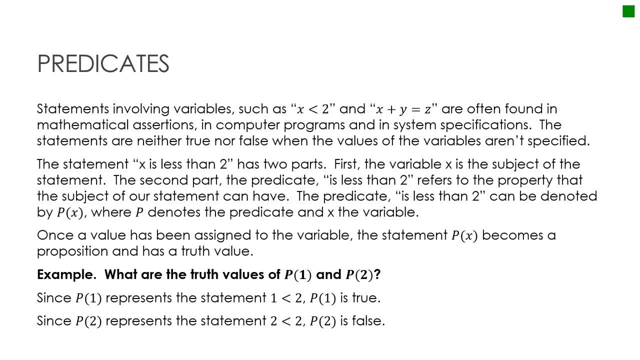 x is less than 2, or x plus y equals z, are often found in mathematical assertions, computer programs etc. etc. And before I actually put a value in for x, those statements are neither true nor false. So the statement x is less than 2 has two parts. We have 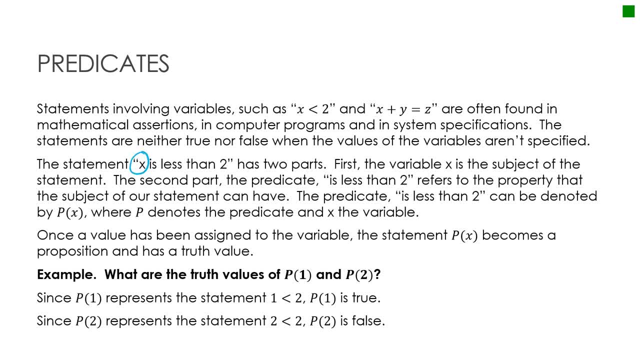 x, which is the variable, and then is less than 2, would be our predicate. It is the property that talks about what is happening with the variable. So we can then say p of x, where p denotes the predicate and x denotes the variable. So once we have p of x, representing x is less than 2,. 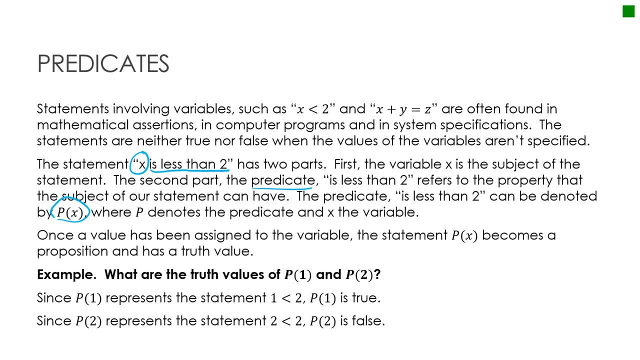 then I can actually look at the truth values. So since p of 1 represents the statement 1 is less than 2, then p of 1 would be true, because 1 actually is less than 2.. If I replace 2, x with 2, then I'd have the statement 2 is less than 2,. 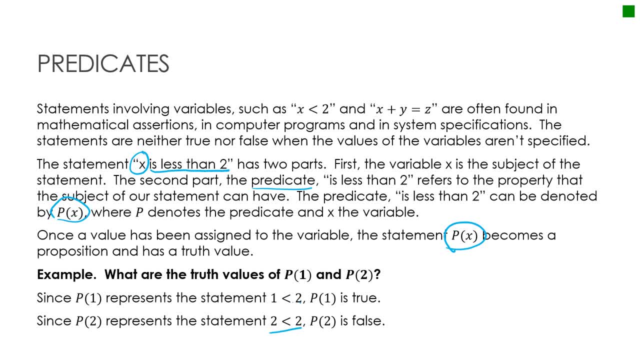 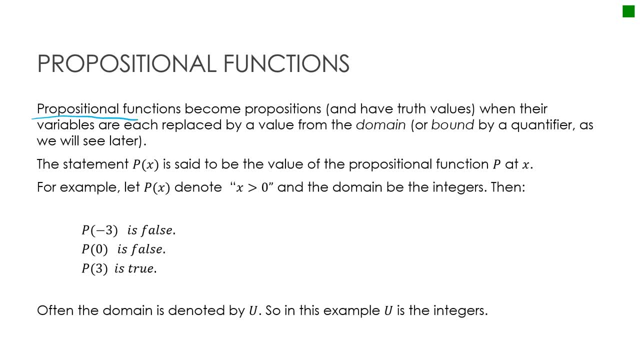 is false. So again the statement p of x is x is less than 2.. So we looked at the propositional function which we called p of x. It becomes true or false again as long as we're replacing the variable by a value from the domain. So domain is going to become very important to us here. 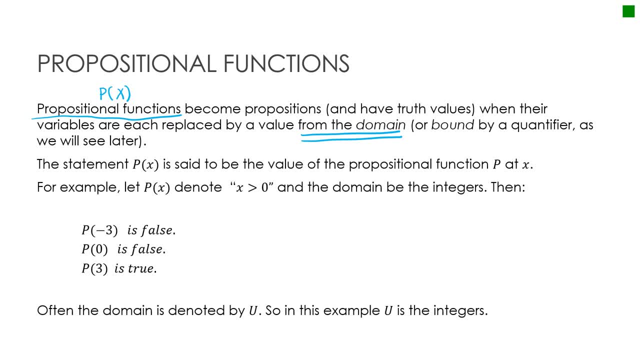 and we'll get to bound by quantifiers later. but it has to be in the domain. So the statement p of x is said to be the value of the propositional function p at x which we just talked about. So for example, let p of x denote x is less or greater than zero and the 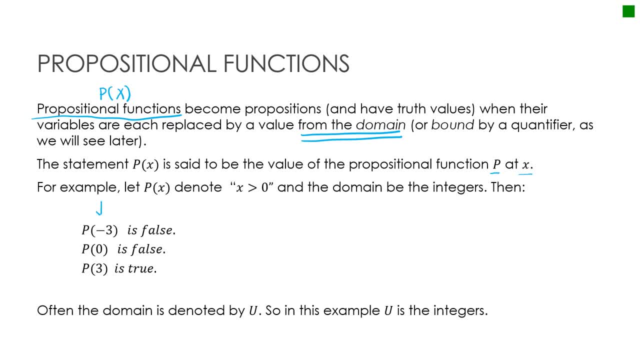 domain be the integers. So notice here: whenever I plug in a value it must be from the integers, which means I couldn't say p of 2.5, since 2.5 is not an integer. it wouldn't work. But we have. 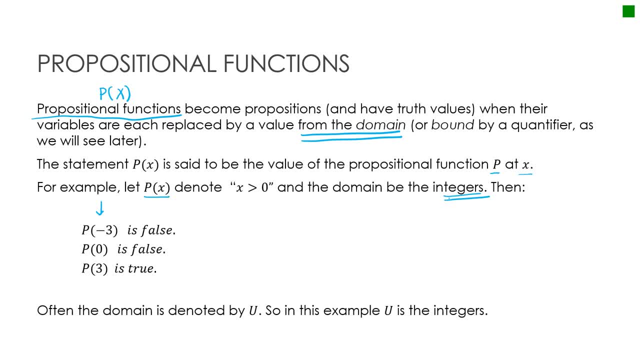 our propositional function p of x denotes that x is greater than zero and p is negative. 3 means negative, 3 is greater than zero, which is why it's false. p of 0 means 0 is greater than 0,. 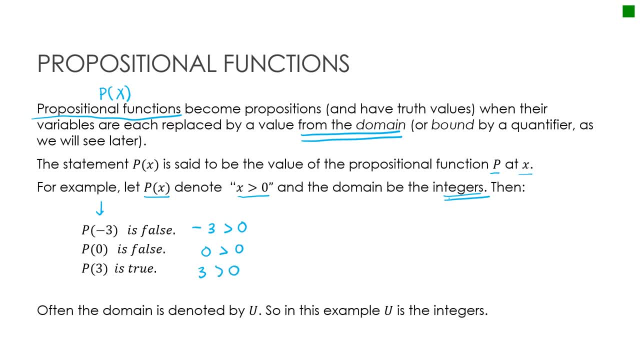 which is why it's false. p of 3 means 3 is greater than 0, which is why it's true. Quite often you'll see the? u, The? u denotes whatever the domain is, and so in this example, u is our integers. 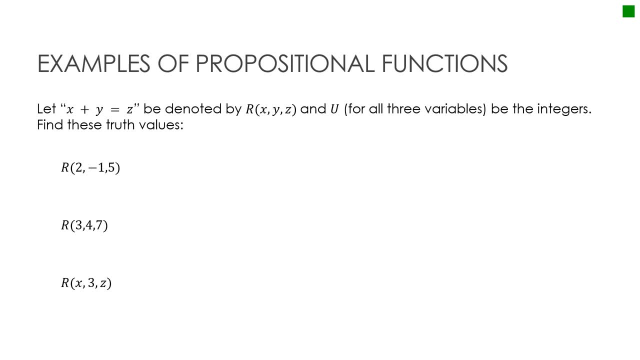 So let's take a look at a few examples of propositional functions and notice I can use a propositional function that has more than one variable. So here my propositional function r has the variables x, y and z and that is representing. x plus y equals z and u for all. 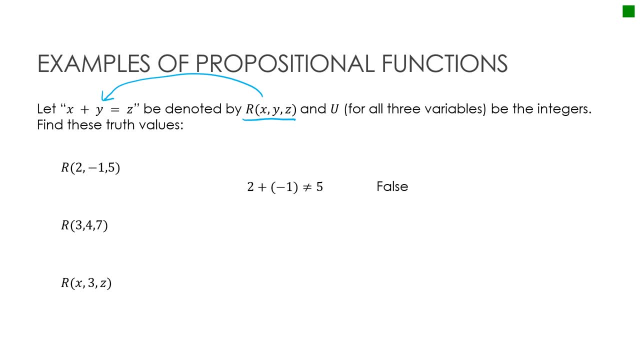 three variables is the integers, which means I have to plug values in as integers. So to find the truth value, I'm looking at r, 2, negative 1, 5, which essentially says that I am equal. sign probably is not appropriate. I'm replacing x with 2, y with negative 1,. 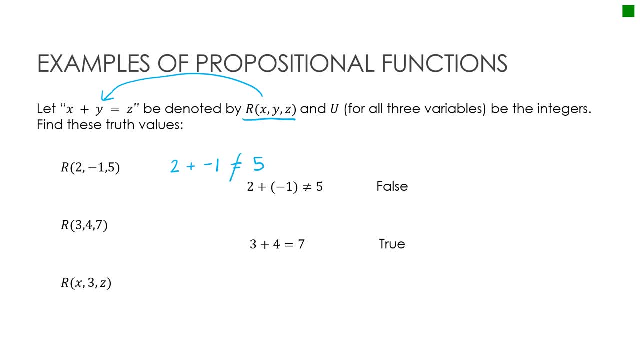 and 5 with z with 5, and notice I get something that is false. so this would be false For the next one. I'm replacing x with 3, y with 4,, z with 7, and z with 5, and z with 7,. 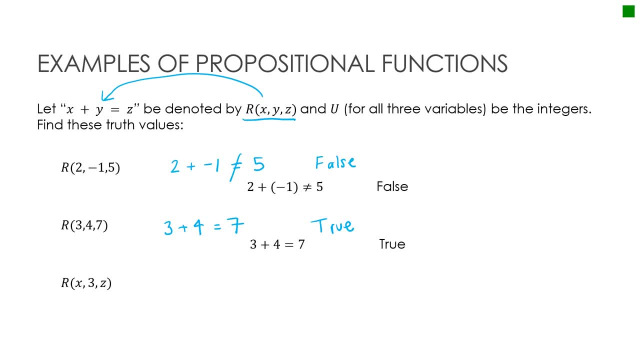 and this is true, and therefore that propositional function would be true. This one: I'm replacing x with x and y with 3, and z with z, and this is not a propositional function, because I need to have values plugged in as integers and that is not what I have here. 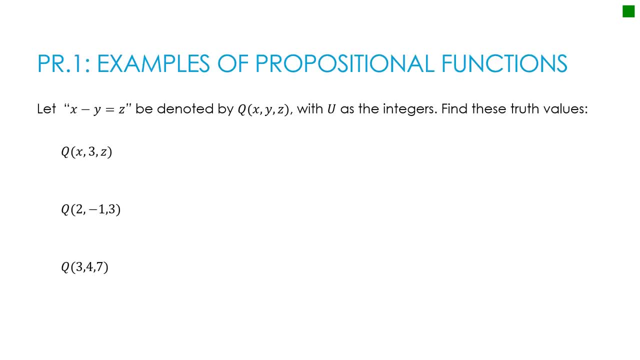 So now I have a jogo. I can claim analysis that qualifies value as 2, and z with 5.. I'm going to refer in puff function to a simple Drag-and-pull function for 서울 jumper, which is true, because nothing wrong with that, and that's why I'm asking you to open up. 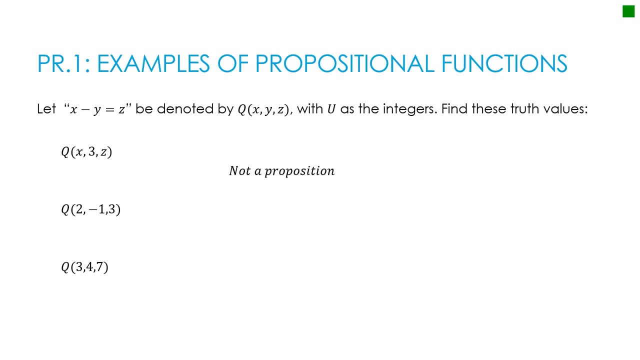 your rounds in the set, and, and so what I'm going to do is I'm going to press right mouse button. I replace x with 2, y with negative 1, and z with 3.. And again I end up with true, because I am. 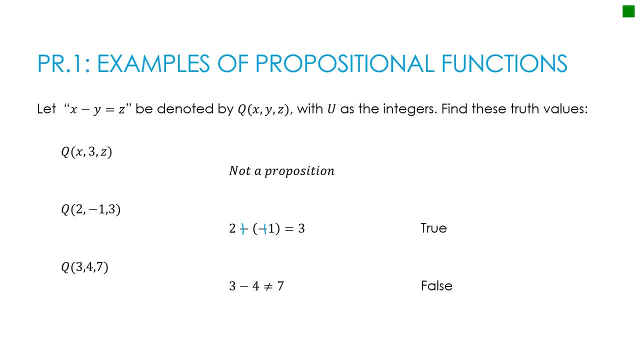 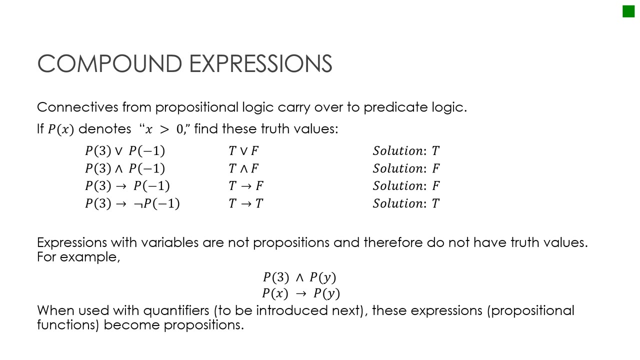 adding 1.. And the last one: replace x with 3,, y with 4, and z with 7.. And that is not true, so that is a false value. In our last couple of chapters we spent a long time talking about. 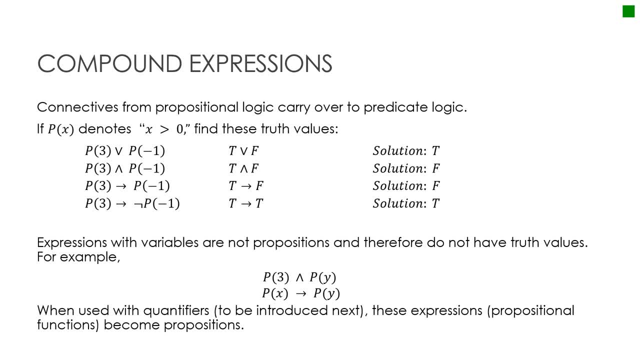 connectives, the disjunctions or the conjunctions, etc. The same ideas carry over to predicate logic. So if I have that p of x denotes x is greater than 0, I can find the truth values, just like I did before. I'm first going to determine if p of 3 is true, which in this case it is. 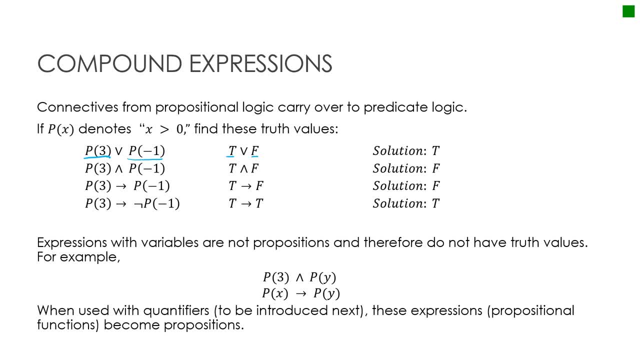 if p of negative 1 is true, which in this case it is not, as it is not greater than 0. And then I'm looking here at an or, and therefore this is true. Same thing for the rest of those. We're really just. 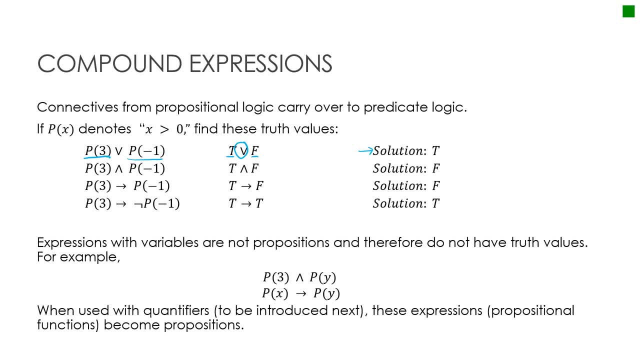 following that same logic that we talked about before, Expressions with variables are not propositions and therefore they don't have truth values, like we looked at on the last couple of examples. So here, if I don't have something to plug in for x or for y, then they're not propositions. 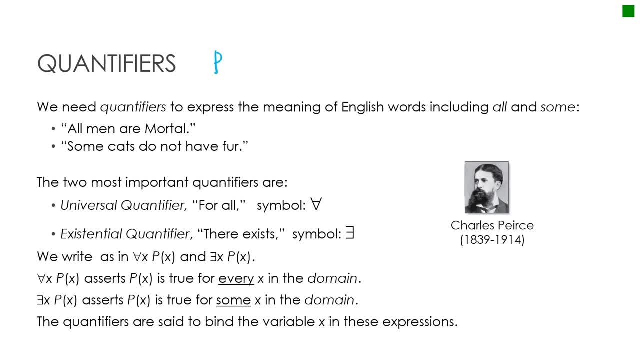 So this brings us to quantifiers, because if we have something like px, where we're not given that x is 3 or 7 or 22,, then we can still consider that a proposition if we have a quantifier. And a quantifier is when we have words like all or some. So let's say x was all of the integers. 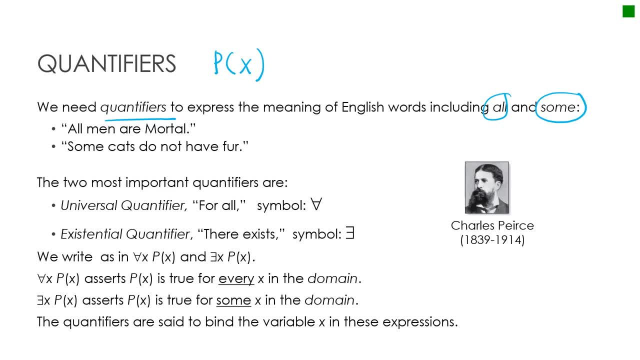 etc. most important quantifiers are for all. which is the symbol, is the upside down A, that's the universal quantifier, and the exponential qualifier is: there, exists, and that symbol is the backwards E. So, for instance, we would write for all x, Px, which tells us that P 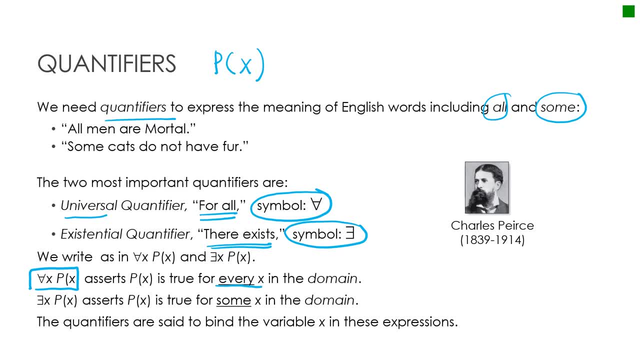 is true for every x in the domain. So for all x's in the domain Px is true. Same thing for there exists. There exists an x, Px tells us that Px is true for some, at least one x in the domain. So these, essentially, are said to bind the variables. So let's look. 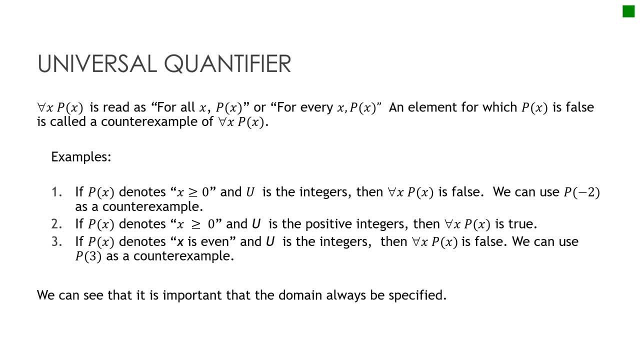 first at the universal quantifier, That is for all x, Px, and again this is how it's read And that essentially means for every x in the domain, whatever the domain is specified to be, P of x is true. So if 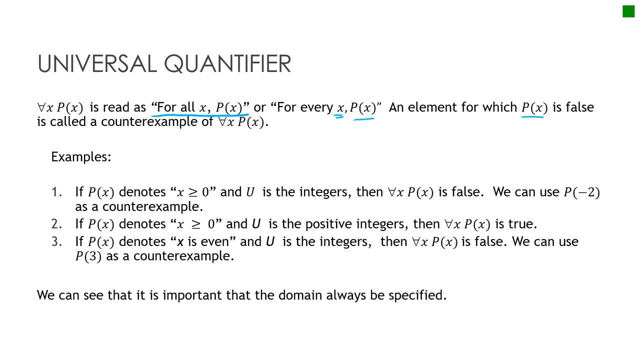 we find an element in the domain for which P of x is false, then we call that a counterexample and essentially we're saying that for all x, P of x is not true by counterexample. So let's look at a couple of examples. 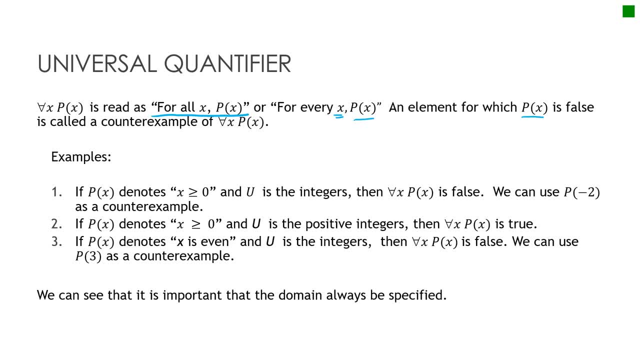 We have. if P of x denotes x is greater than or equal to zero and u, being the universe, is the integers, which means positive and negative whole numbers, then I can tell right away that I can use a counterexample of say negative two and negative two makes 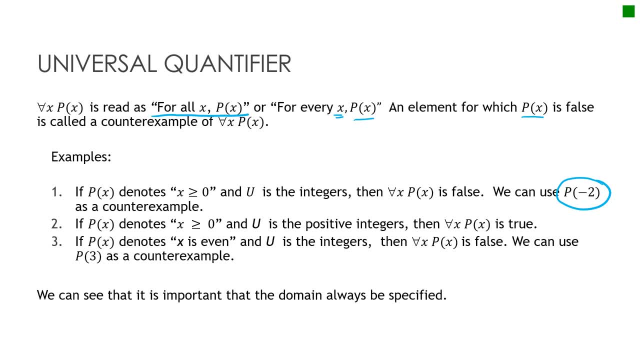 this statement not true, because negative two is in the universe of integers. then for all x, Px is false. I counterexample In the same way. now we're looking at the same, x is greater than or equal to zero and we're saying u is the positive integers. so now we're starting at zero and working our 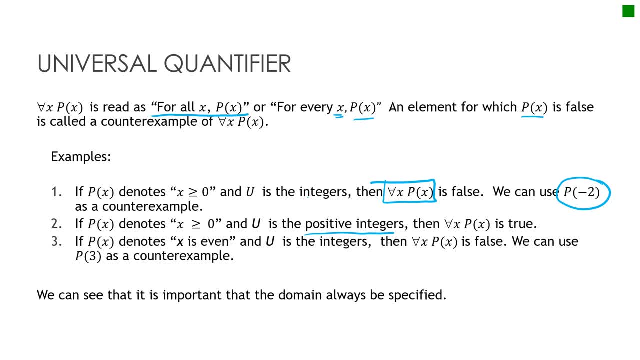 way up and let's look at the lowest one. Yes, this makes the statement true. All of the other values will be higher than that. so still true, and therefore for all x, P of x is true. If P of x denotes x is greater than or equal to zero, then we're saying u is the positive. 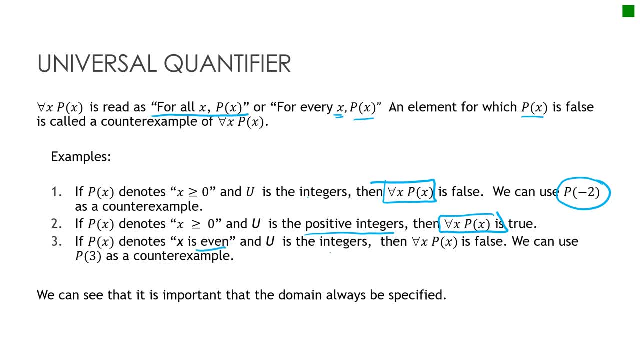 integers, which means that we're going to have to counterexample all the way to the original one. if we want to counterexample all the way to the original one, But if t denotes that x is even and u is the integers, then obviously we can come up. 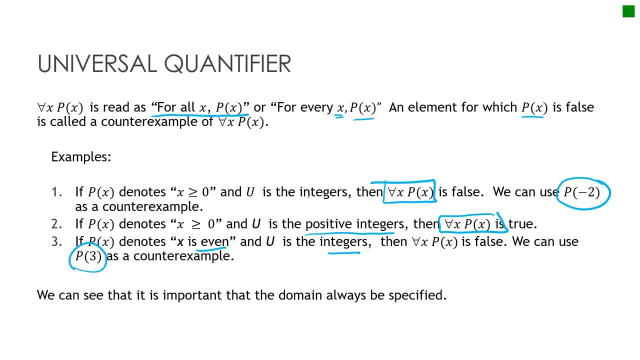 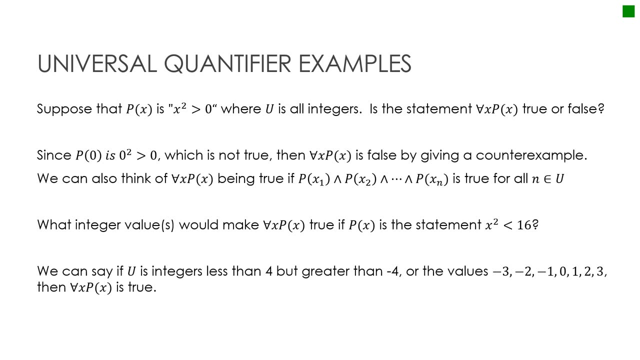 with a counterexample, because P three or P one, etc. would be counterexamples. So just remember that the domain, or whatever the domain is, is important. Let's look at a couple of examples for the universal quantifier. Suppose P of x is x. 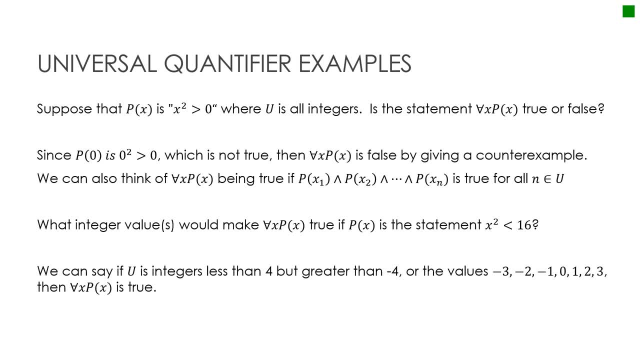 squared is greater than zero. where u is all integers, Is that the same as p of x? Is that the same as p of x? Is that the same as p of x? statement for all x, p, x. true. So again, the domain is all integers. So is it true that whenever we 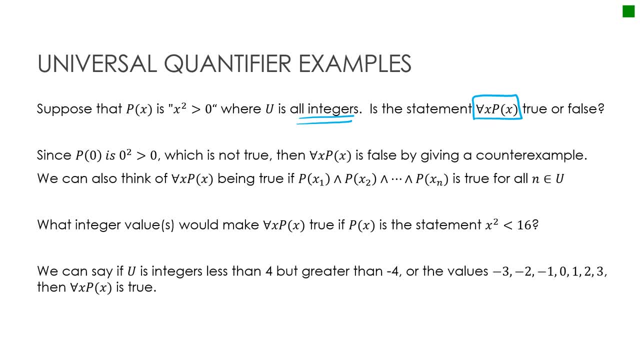 square an integer, it will be greater than zero. Well, almost, but if I plug in zero, p of zero, that would be zero. squared is greater than zero, which is not true. So, essentially, for all x, p of x is false by giving a counterexample. So essentially, we're thinking about this being true if for every 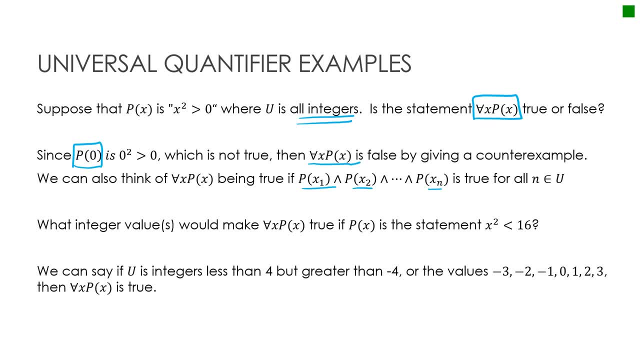 single item. I can plug in for x1 and x2 and x3, etc. everything has to be true. Next practice: what integer value or values would make for all x p of x true if p of x is the statement x squared is less than zero? So is it true that for all x, p of x is true if p of x is the statement x squared is less? 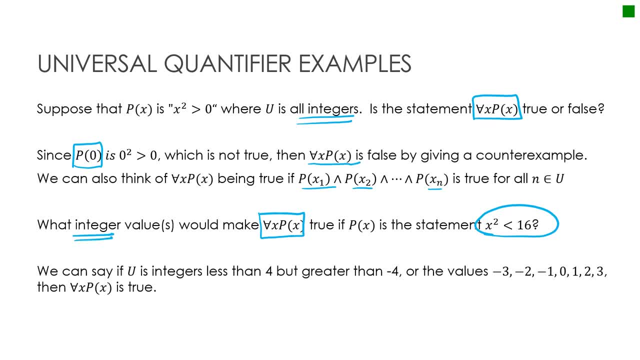 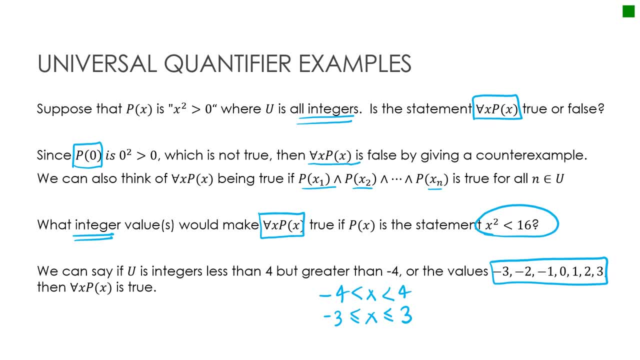 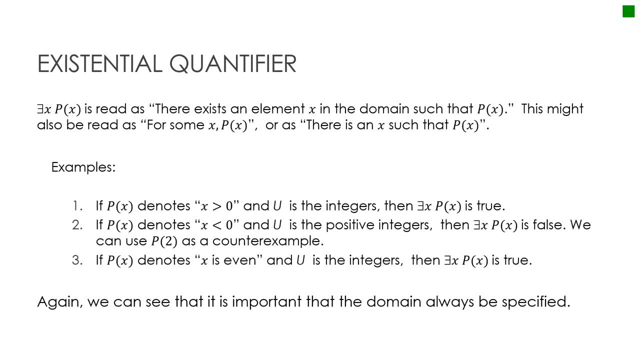 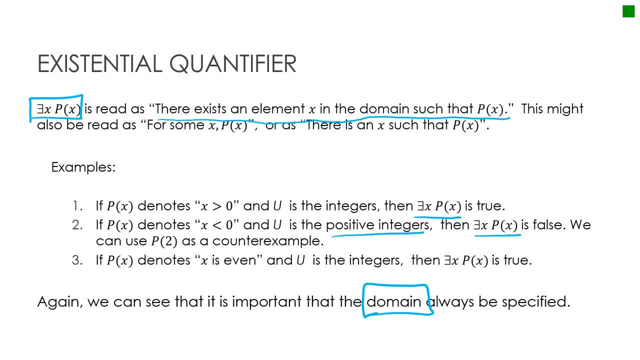 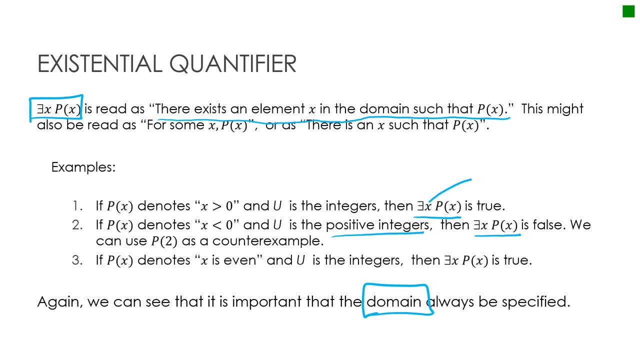 counterexample like negative 1, that is a counterexample However I'm looking for. there exists. So as long as something exists, then we have proved it. If px denotes x is even and u is the integers, so I can say there exists some x, p of x is true. So again, this is different. 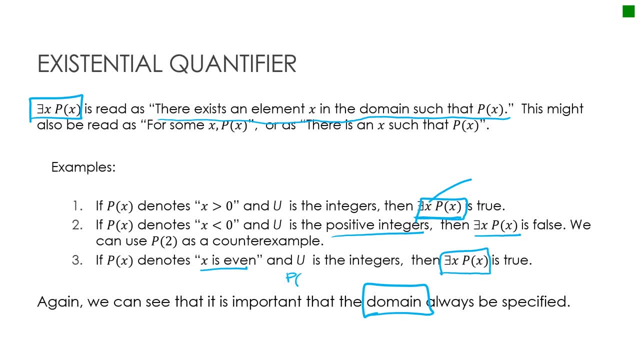 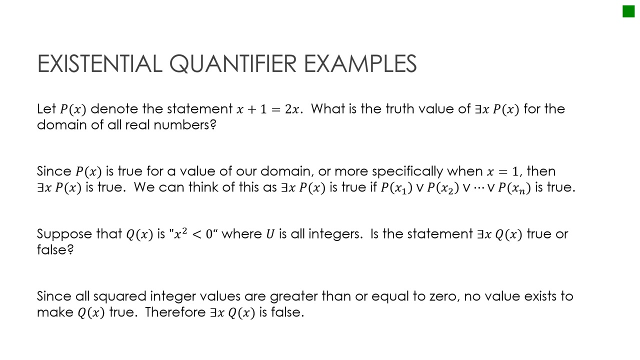 It's okay to have p of 3,, which is a counterexample, because all I need to show is p2,, which is an integer, that is, even that shows there exists. So again, the domain is very, very important to us. Let's look at a couple of practice for the exponential qualifiers. 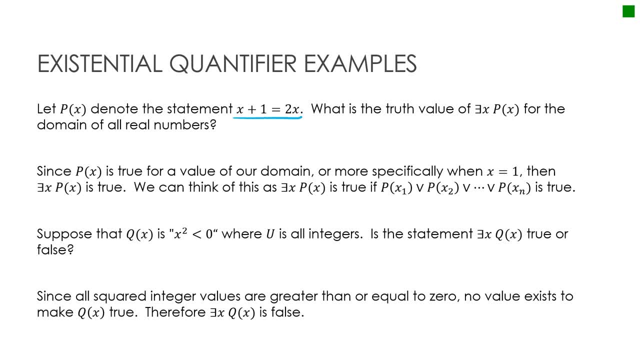 So let p of x denote the statement: x plus 1 equals 2x. What is the truth value for? there exists x and x? p of x for the domain of all real numbers. So if the universe is all real numbers, then what is the truth value of? there exists an x px. 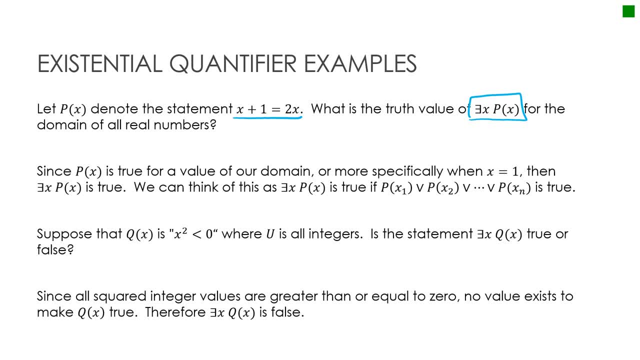 So in order for there exists that to be true, we just need something to be true. So in this case, I could subtract x from each side and get 1 equals x, And so I know that if I plug in the value of 1, then there exists an x. p of x is true, because all I need is just 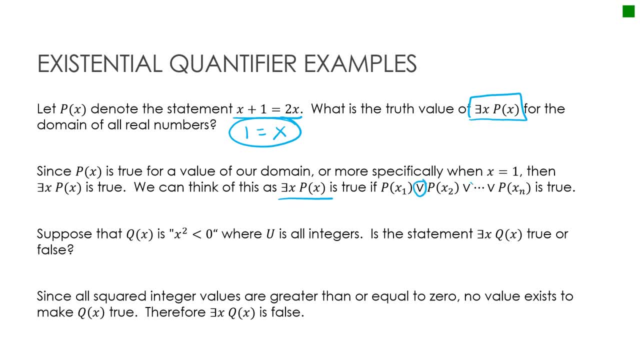 1. And again there exists- we're talking about: this is true or this is true, or this is true, etc. Suppose: q of x represents x squared is less than 0, and u is all integers. Is the statement there exists an x, q of x, true or false? So, essentially, 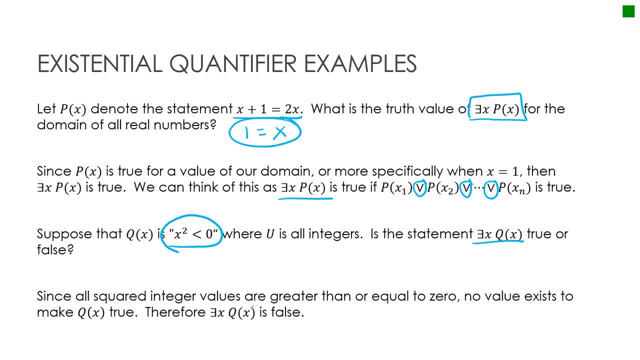 what we're saying in English is: is there an integer, at least one that I could plug in, for x, that it would be less than or equal to 0?? And in this case, nope, we're dealing with integers. 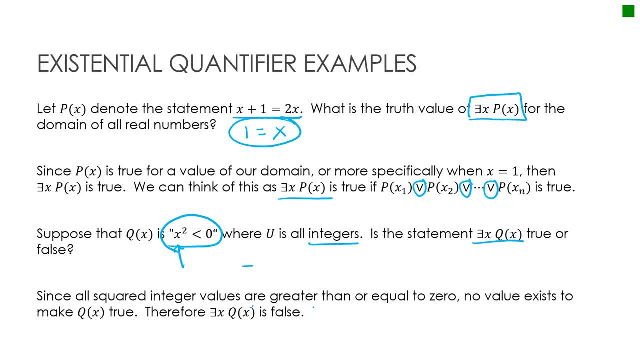 And no matter what integer we put in there, if it's a negative integer, it is not less than 0.. If it's a positive integer, oops, it is not less than 0.. If it is 0 squared, it is not less than 0.. So there's no value that exists. 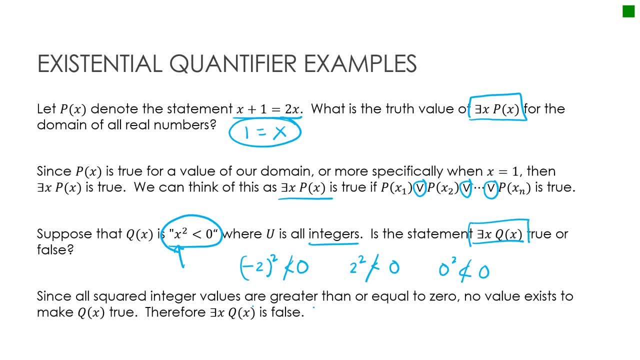 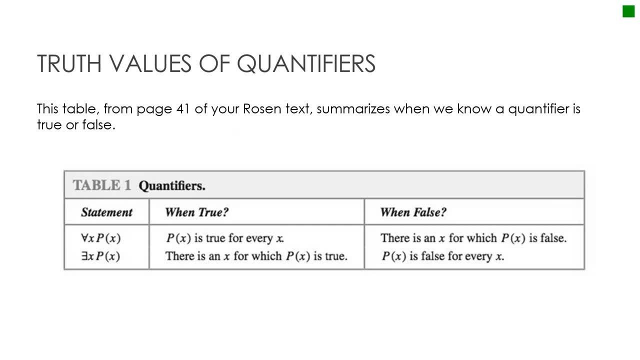 And therefore this statement is false. There exists an x, q of x is false. So, again, if we are asked to prove if the statement is true or false for all x, p of x is true when p of x is true for every single x in the domain. 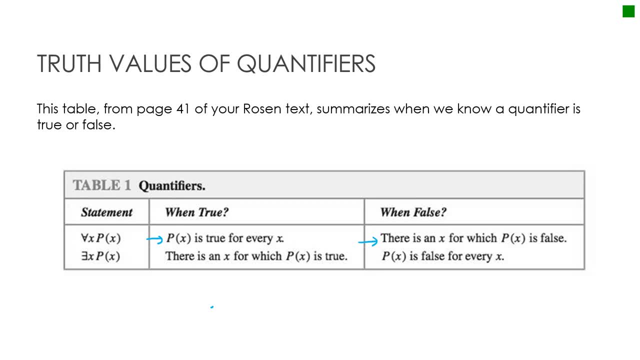 But if there exists an x for which it is false, then we say that the whole statement is false, For there exists an x, p of x. it's true if we can find at least one x for which p of x is true. 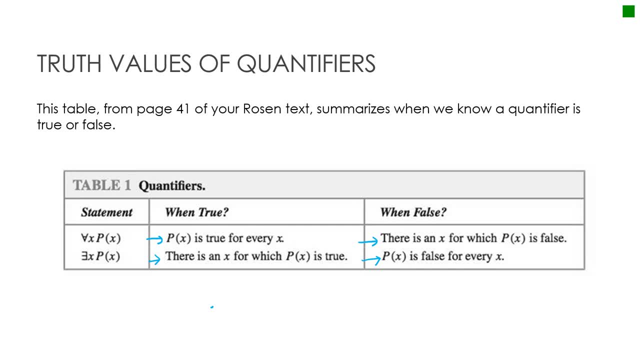 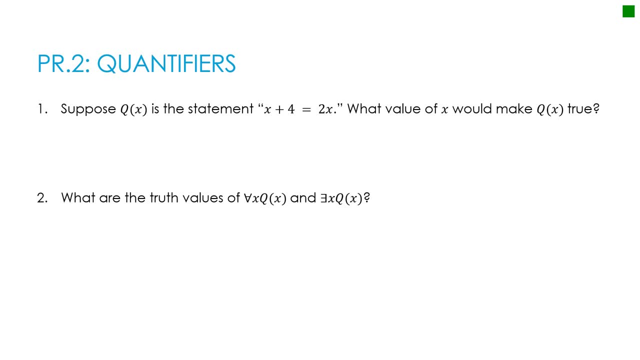 It's false if it's false for all x's. So you can see how they're sort of opposites of one another. So here's a practice question for you to try, two in fact. So I'd like you to do both of these questions and then press play to see how you did. 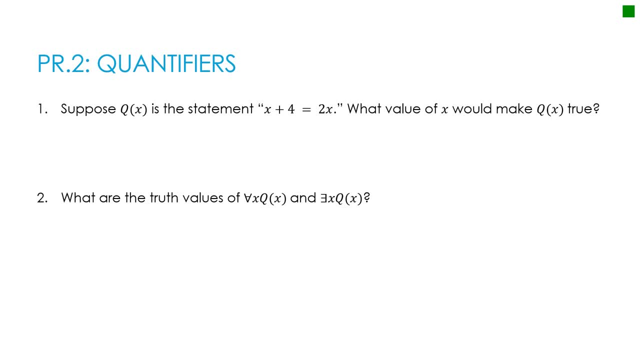 So the first part pretty straightforward, just basic algebra. Suppose: q of x is the statement x plus 4 equals 2x. What value of x would make q of x true? And so we can just solve it as we normally would subtract x from each side. 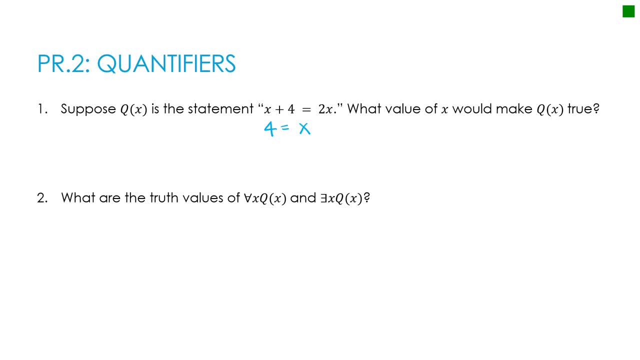 and I would get x equals 4.. That would make the statement true. So what are the truth values of for all x, q of x, x, and there exists an x, q of x, So q of x, we know, is only true when x is equal to 4.. So there, 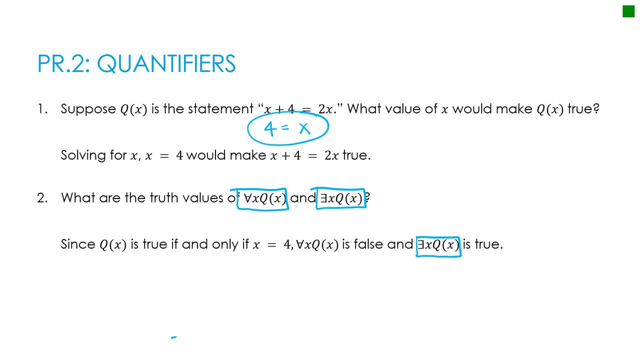 exists an x, q of x is true. We're not specifically given what the domain is here, but assuming the domain is all real numbers or even all integers, we can easily see that this would be false, because there are so many values that I could plug in like, say, 2, that would make this statement. 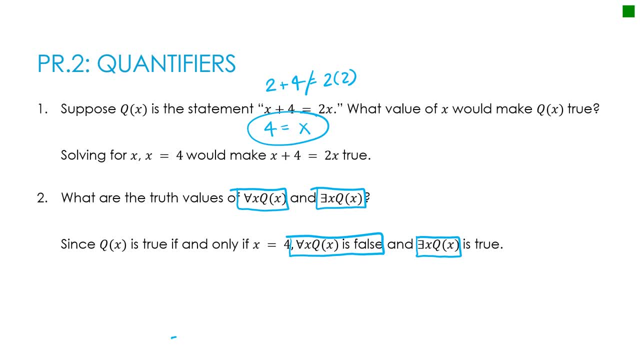 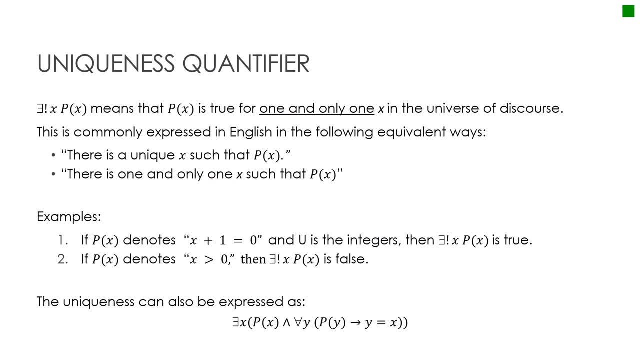 false. Therefore, it's true, for there exists, but not for for all. One last quantifier to talk about, although there are so, so many, but just to throw this one out there as well, that you might see, this is the uniqueness quantifier. It's very similar to there. 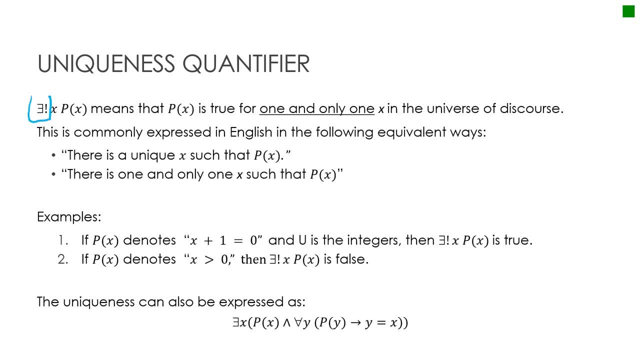 exists, but in this case- and again note the notation here- it means there exists a unique. So basically we're saying there is only one value in the universe of discourse or the domain that makes the statement true. So if p of x denotes x plus 1 equals 0 and u is the integer. 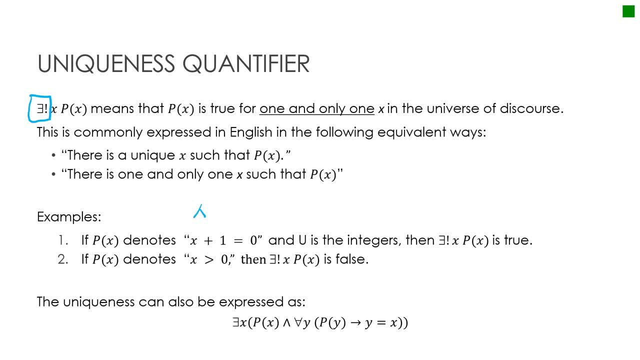 we could solve that by subtracting 1 from each side and getting x is negative 1.. So there's only one solution and therefore there exists a unique x. p of x is true. However, let's say we have p of x denotes x is greater than or equal to 0, again using u as the integers. Then we're saying: well, 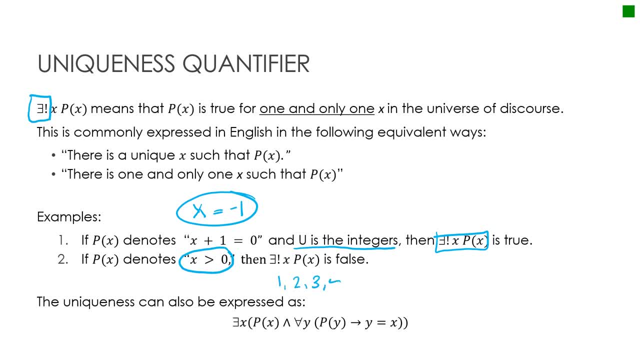 I could plug in 1 or 2 or 3.. Or 4 or 5, etc. etc. etc. So there exists plenty, but does there exist a unique? No, Therefore there exists a unique x. p of x is false, And here is just another notation that we could use. 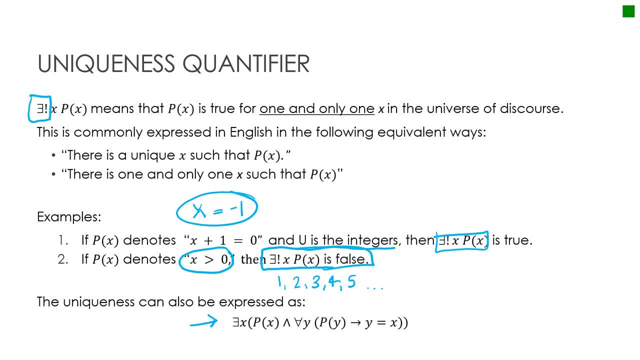 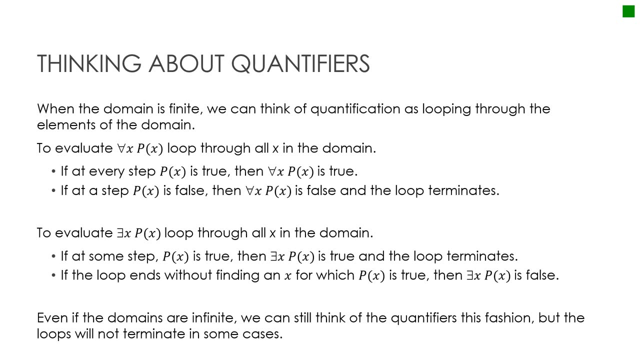 as we get more and more into all of the different things that we're going to learn about. This is a way that you might see. there exists a unique expressed in a different way. So, as we're thinking about quantifiers and we have a domain that is finite, meaning not continuous. 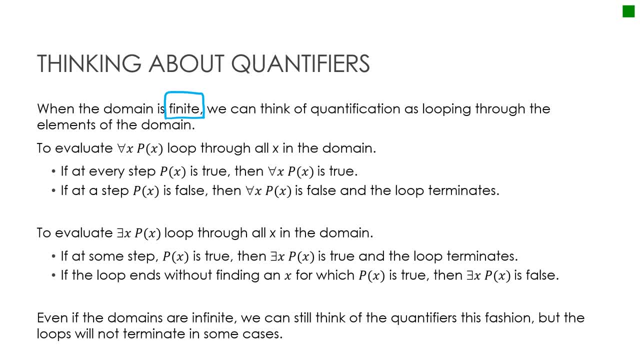 doesn't go on forever, etc. we can think of quantification as looping through the elements of the domain. So let's say the domain is 1,, 2,, 3.. I would check p of x for 1, and then for 2,. 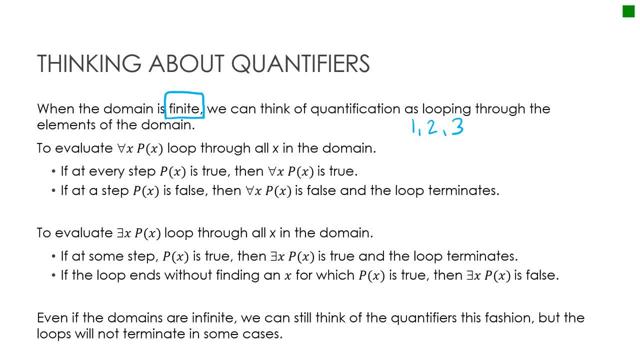 and then for 3.. And assuming that those are all true, then for all x, p of x is true, And then for 3, p of x is true. However, if I get to one that is false, then the loop terminates and therefore. 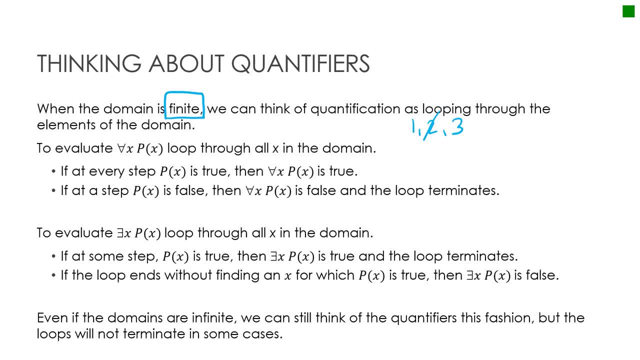 it's false. So to evaluate there exists. again, we're looping through all of the elements of the domain, say 1,, 2, 3. Once we get to a point where p of x is true, then we know that there exists. 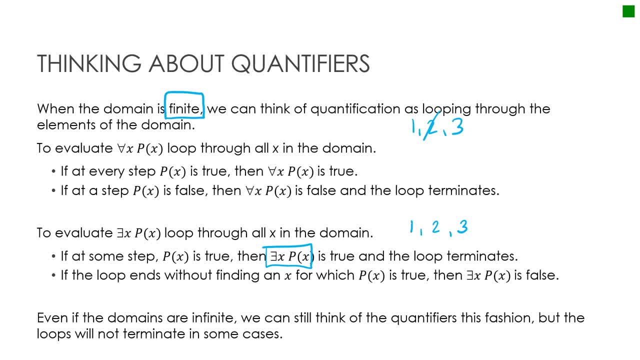 an x, such that p of x is true. For instance, let's say 1 was false but 2 were true. Well, I can stop checking, because I know that there exists a unique x. p of x is true If I've made it all the way through my list and none of them were true. 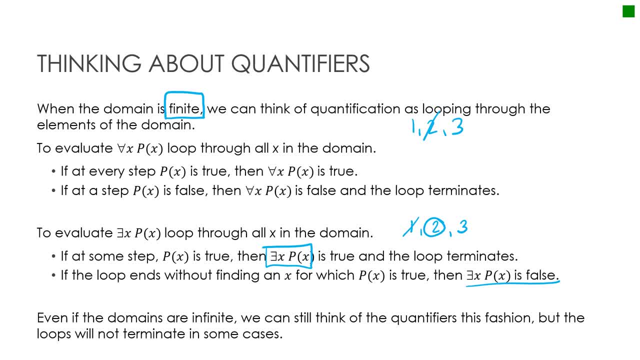 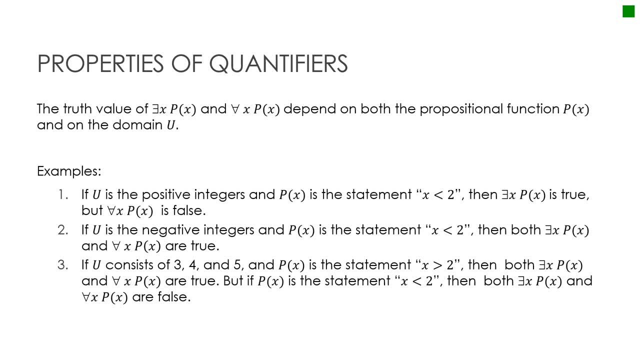 then obviously there exists an x. p of x is false. Again, not to beat a dead horse, but you know it's so important that you understand what the domain u is for each question that you're working on. So here's a few examples. 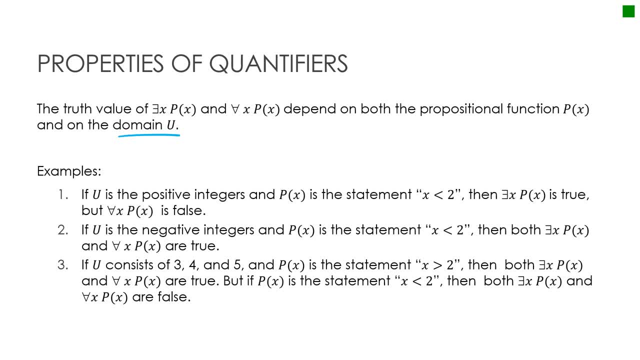 Let's say u is the positive integers and px is the statement x is less than 2.. Then there is a positive integer, such that x is less than 2, because 1 is less than 2.. But for all of x, p of x is false, because if I could use 2, that is false. 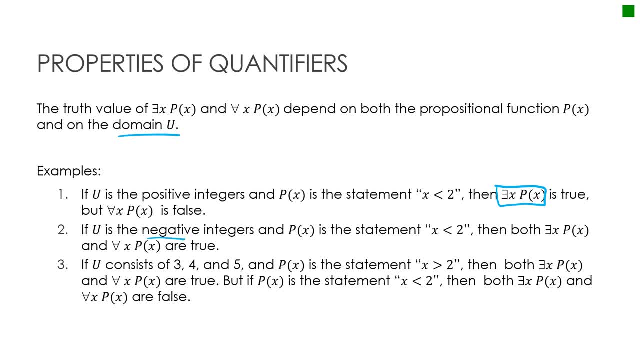 If u is the negative integers, then the statement x is less than 2 is true for both there exists an x. p of x is false because, let's say, negative 1. Negative 1 is less than 2. And there are no values that make it false in the negative integers and therefore both there exist. 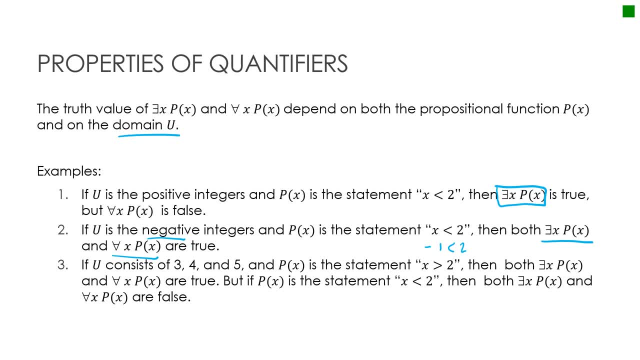 and for all is true If u is 3,, 4, and 5 is the universe and p of x is the statement, x is greater than 2, then everything's true, because 3,, 4, and 5 are all greater than 2.. But if it's less than 2,, 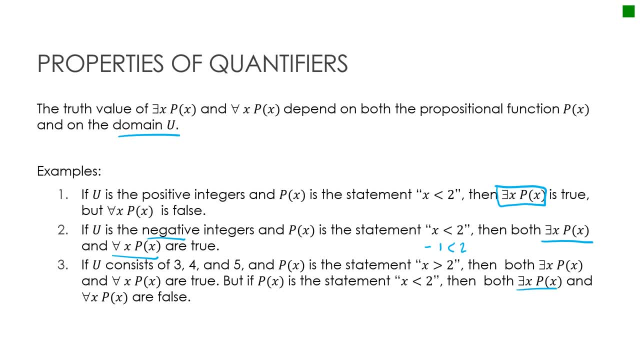 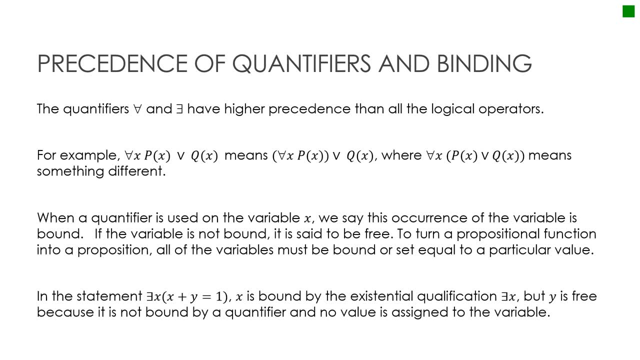 then both of them are false, Because there does not exist one, and certainly not all of them. So let's talk a little bit about the precedents, or essentially, like the order of operations of quantifiers. We know that for all and there exists. both have higher precedents than all of 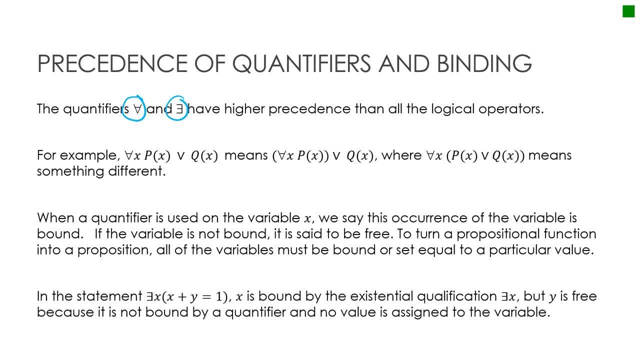 the other operators. So, for example, in for all x, p of x or q of x, means that there is no correct answer to the squared root of x, p of x or the squared root of x. This means that the for all. 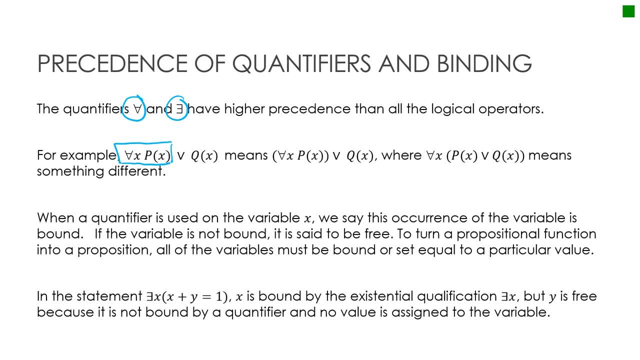 is only on the p of x and not on the q of x. So think of those as joined together. What a quantifier is used on the variable? we say that it is bound, So the quantifier being at least three or, you know, at most seven or whatever. 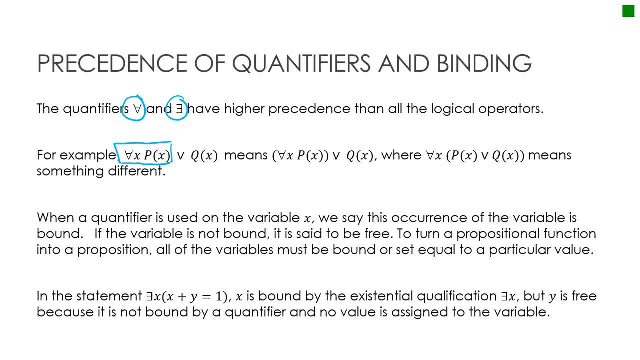 If it's not bound, it's said to be free To turn a propositional function into a proposition. we must either bound them or set them equal to a particular value. So, again, in order for it to be a proposition, we either have to say okay, we're doing p of three, or we're saying for all. 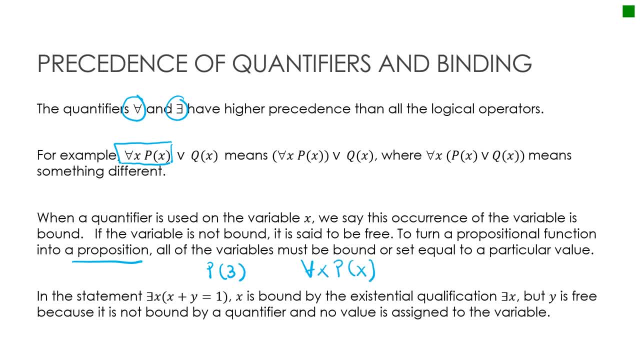 x, p of x. where, say, the universe is? integers. So we must essentially assign a value or values to a propositional function in order to turn it into a proposition. Here's a good example: down here In the statement there exists an x. 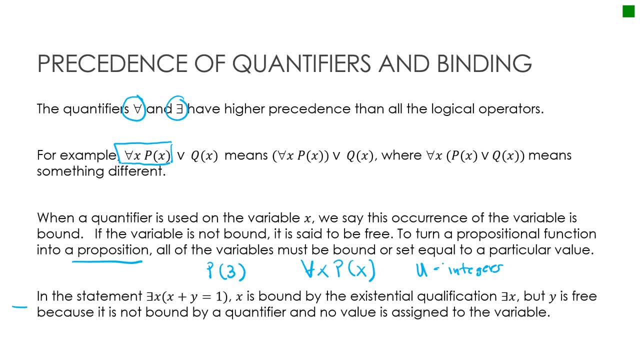 such that x plus y equals one. x is bound by the existential qualification. there exists an x, but y is free because it doesn't say what y is and it doesn't bind it in any way by saying there exists or for all, etc. because we don't have a value assigned to the variable. 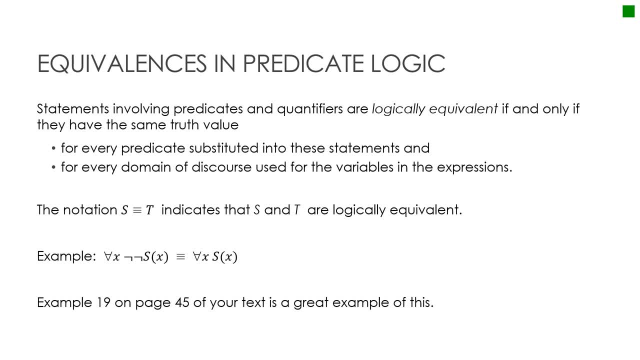 In section 1.3, we spent some time talking about equivalences, logical equivalences. Same holds true for predicate logic For predicate predicates and quantifiers are logically equivalent if, and only if, they have the same truth value. So the same way we did it before when we made a truth. 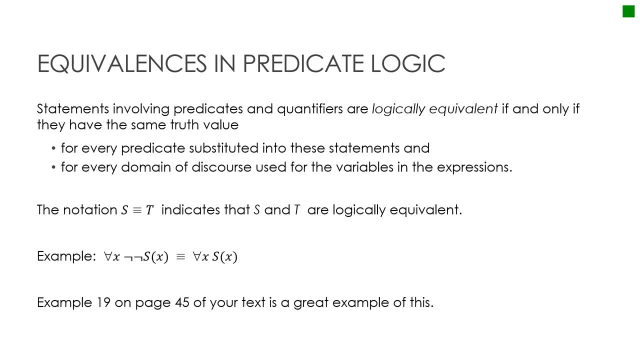 table, etc. Here we're not necessarily creating truth tables, but essentially we're saying: using that same value, we're creating a truth table, etc. Here we're not necessarily creating truth tables, etc. Here we're saying: using that same value, we're creating a truth table, etc. 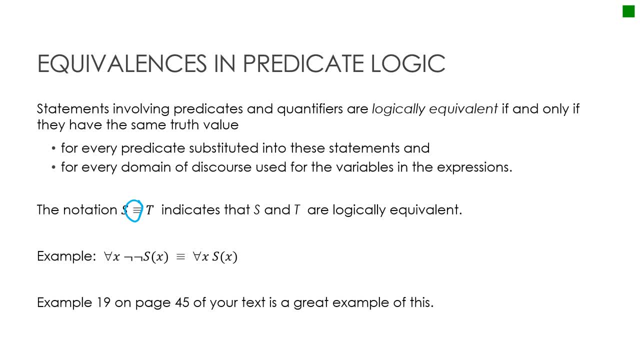 notation saying they're logically equivalent. So for all x, not not s of x, is equivalent. again, using that double negation law is equivalent to for all x, s of x. Page 19, or example 19,- excuse me, on page 45 of your text is a great sort of a longer example of that. 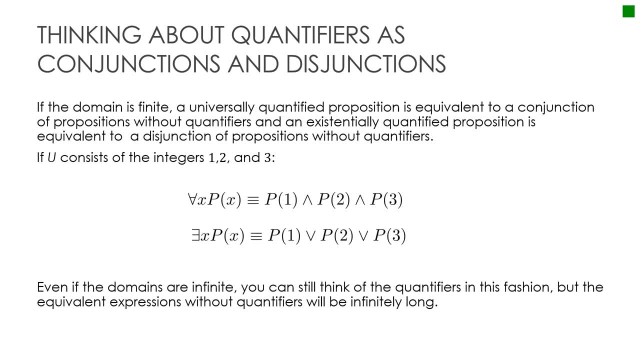 As we first learned about quantifiers. we did talk about this a little bit, but I just wanted to make sure that this distinction is clear. If I'm talking about a for all, x, p of x, essentially I'm saying that p of 1, and p of 2, and p of 3, and 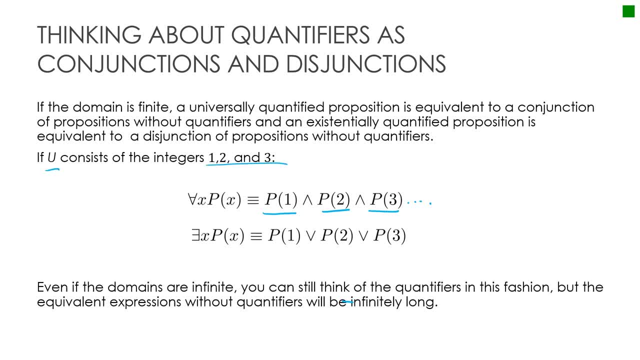 depending on what the domain is. so here we're saying u consists of 1,, 2,, 3, but let's say u consists consisted of the positive integers, then p of 1, and p of 2, and p of 3,, etc. 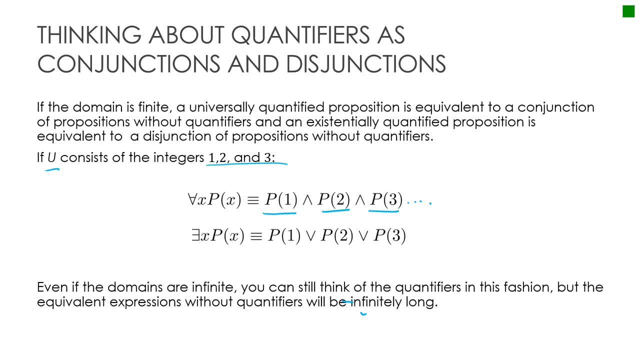 all the way up to 1,, 2,, 3,, etc. all the way to, you know, p of n, whatever the endpoint is, say, all the way up to 22,. well then, this would be 22.. All of those would have to be true for all of x, p of x, to be true. 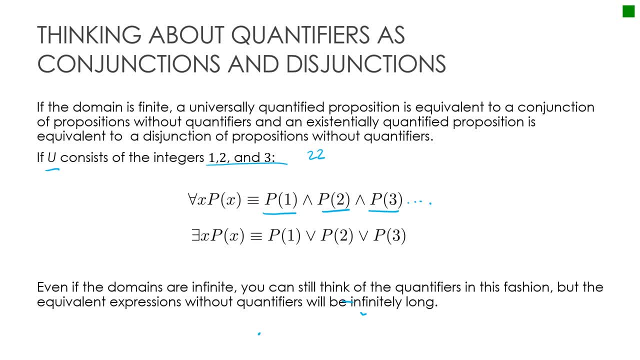 Similarly, if we're talking about the exponential qualifier, basically saying there exists, it has to be or p of 1, or p of 2, or p of 3, etc. etc. etc. must be true in order for that to be true. 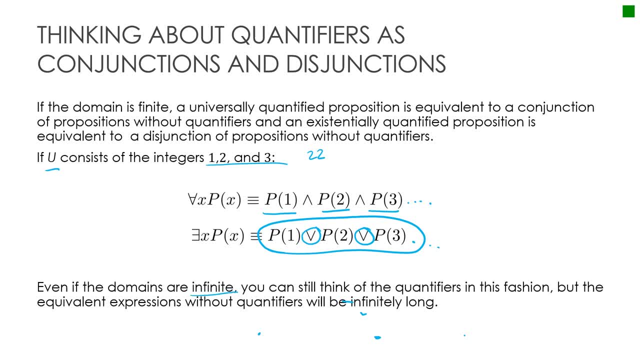 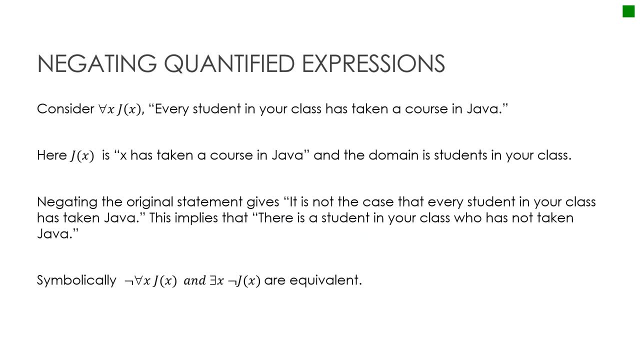 And again, you can certainly do that for an infinite domain. you would just have to keep writing and writing and writing and utilize your ellipses. So, now that we're hopefully a little bit more familiar with quantifiers, let's talk about how to negate a quantified expression or an expression that contains. 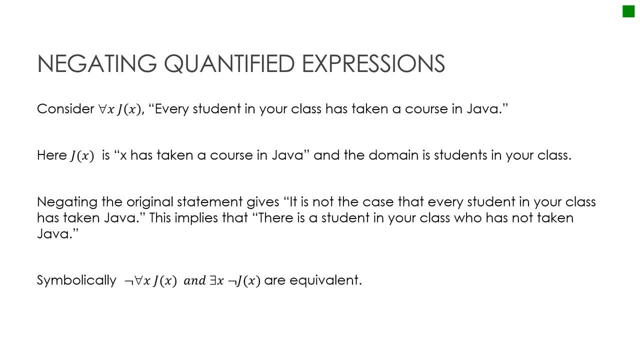 a quantifier. So consider for all x, j of x. Every student in your class has taken a course in Java. So j of x here is x. whoever the domain person within the domain is has taken a course in Java and the domain is, say, students in your class. So if we negate the original statement, 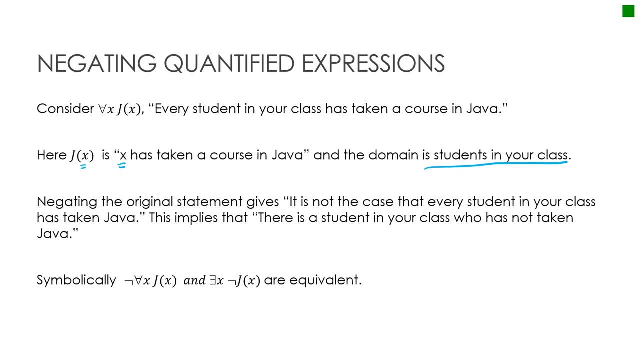 we're basically saying it's not the case that every student in your class has taken Java, or there is a student in your class who has not taken Java. So symbolically, we're saying not for x, j of x, we're saying that every student in your class has taken Java. 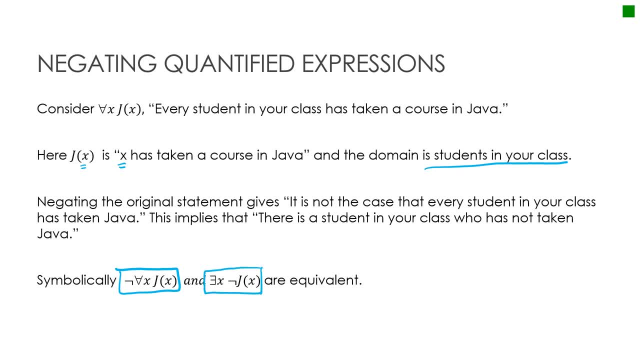 So we're saying so for all x, j of x. that means there exists some person in your class who has not taken Java. Those two things are equivalent. So again, just like when we negated a conjunction, we got the disjunction of the negations. this is sort of the same concept We're saying if we're 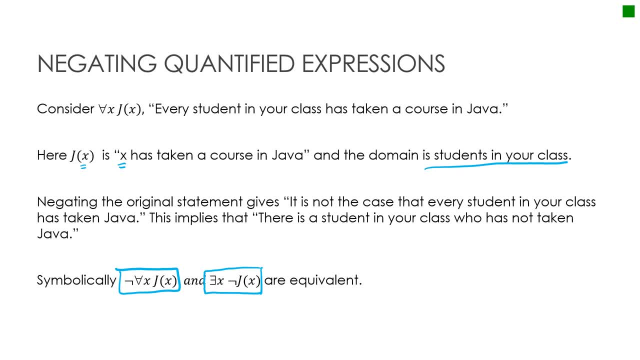 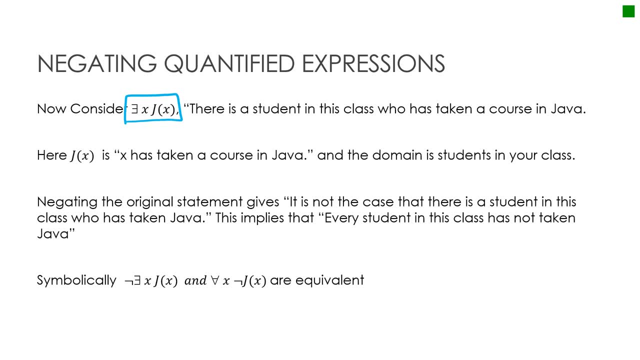 if not all that means there exists some person that is not, and similarly, of course, if I have, there exists an X, J of X, or there is a student in the class who has taken a course in Java. J of X would represent X has taken. 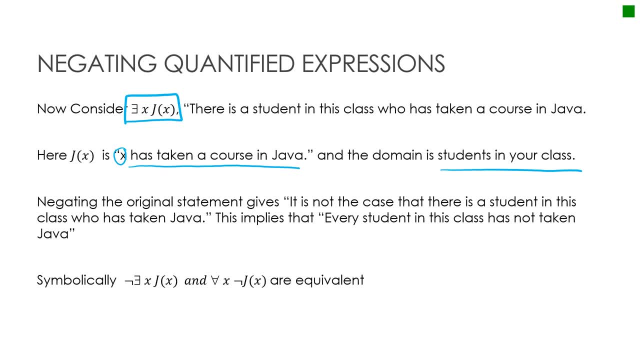 a course in Java, the domain students in your class. if we negate it, we're saying it's not the case that there is a student in this class who has taken Java, or essentially every student in the class has not taken Java, and so we can say symbolically that there does not exist an X, J of X. then that is the same. 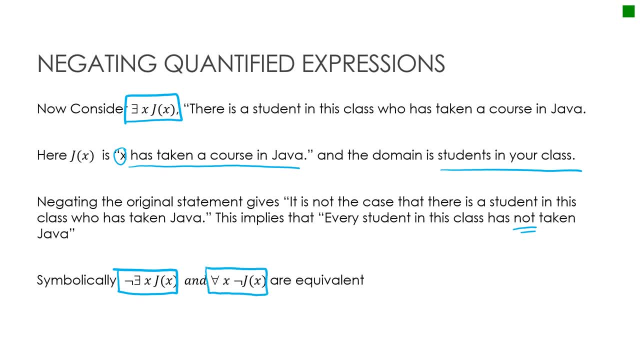 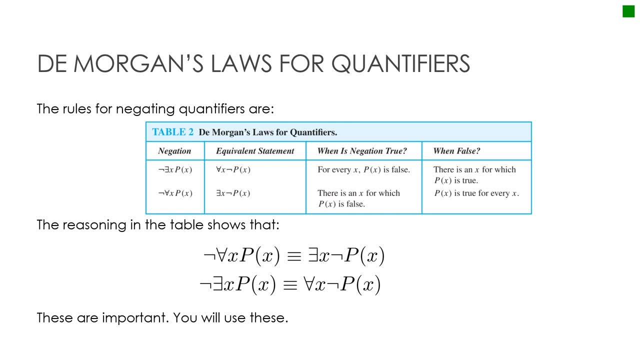 as saying for all of X, not J of X, is true, those two things are equivalent. this table essentially just is a nice summary of what we just talked about. so if we negate there exists, it's for all there does not exist, etc. so these are important. make sure that you understand them, just like de morgan's laws. 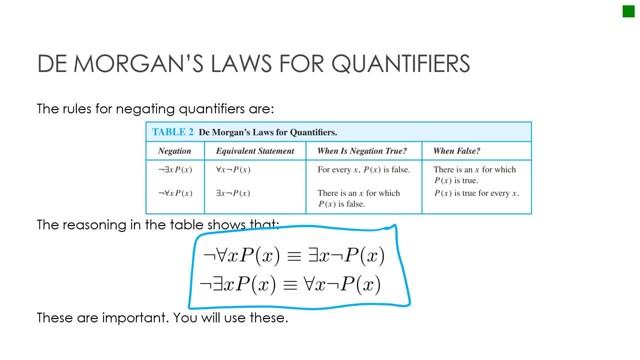 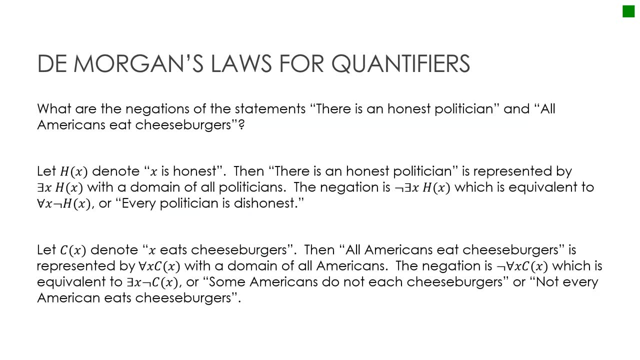 it's the same idea. we're going to use them all of the time. this is de morgan's law for quantifier. so let's do a little bit of practice for de morgan's laws for quantifiers. so we want to negate the statements. there is an honest politician and all americans eat. 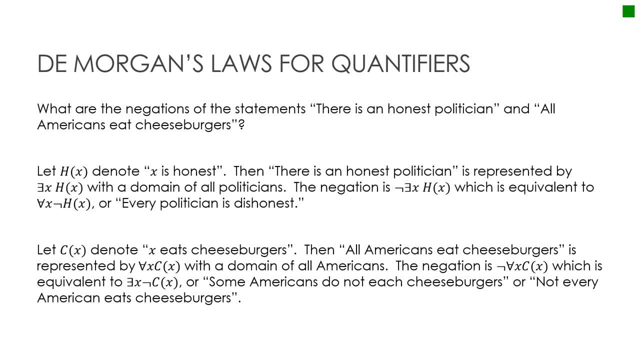 cheeseburgers. so again, we're just going to use de morgan's law. just like before, we're going to take a look at our original statement and we have to write it, in this case using a quantifier, and then we're going to negate that quant- uh, quantified statement. so let h of x denote that x is honest. 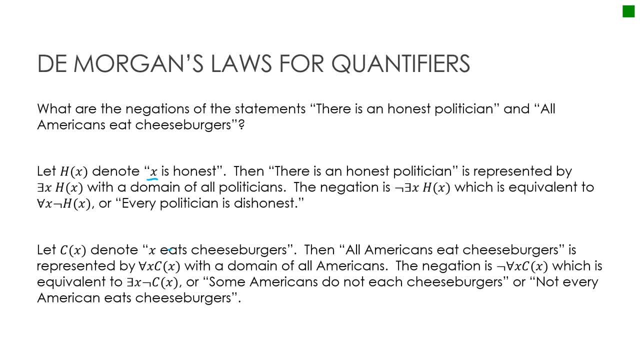 then there is. there is an honest politician. there is an honest politician is represented by there exist in x, h of x, assuming that the domain is all politicians. if i negated the there exists, it is equivalent to for all x, not h of x. so if i negate, 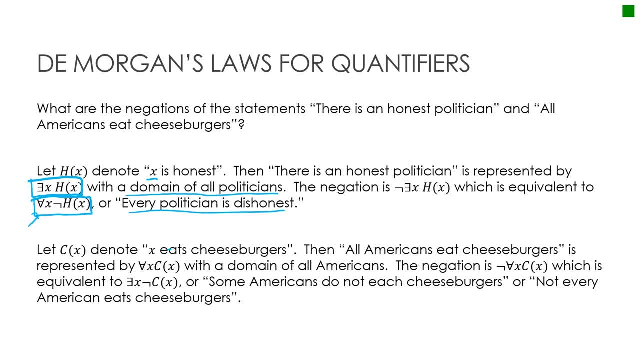 it. i'm basically saying every politician is dishonest, so for all politicians h of x is not true, meaning they're all dishonest. same idea for all americans eat cheeseburgers. so if all americans eat cheeseburgers, we could write that as a x for all x. 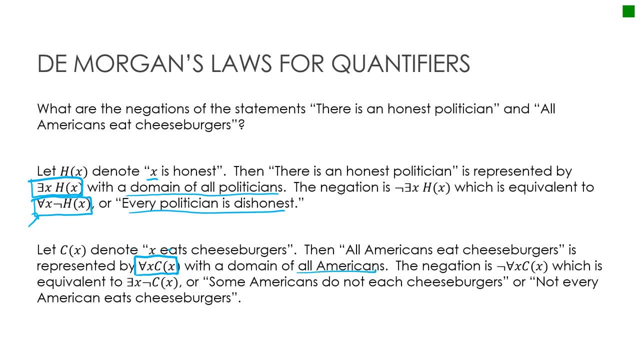 c of x. the domain is all americans, because that is what it's given to us in the question. the negation would be: not for all x. c of x, which means there exists some x such that c of x is not true. so some americans do not eat cheeseburgers, or not every american eats cheeseburgers. 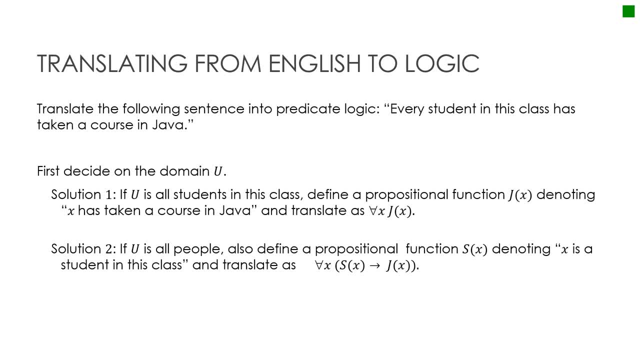 now, as i've said so many times throughout this video, the domain is super important. so the way that you write the domain might change, or will change the way that you're going to write the sentence into predicate logic. so let's say, each or every student in class has taken a class. 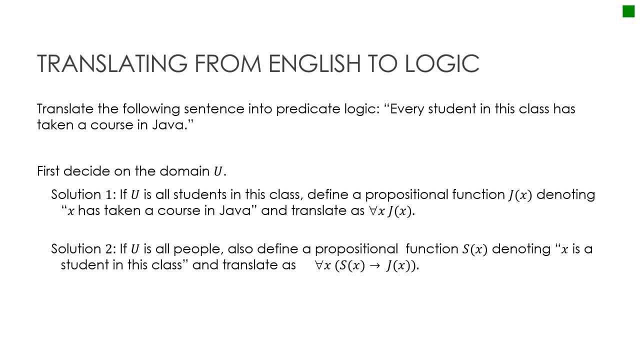 taken a course in Java. well, if U is all students in the class, that kind of takes care of this and we're just saying all students have taken a course in Java. so for all X, which means for all students in the class, for all students in the 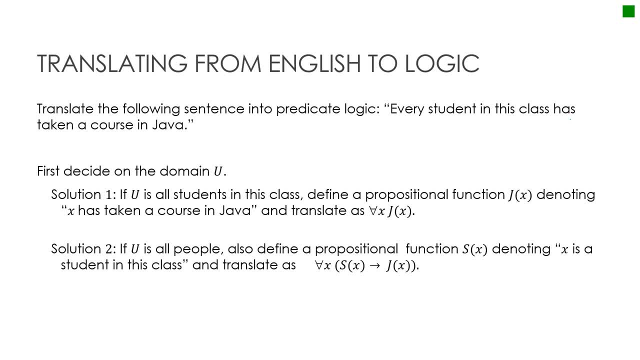 class. they have taken a course in Java. however, let's say I do not write it that way. let's say the universe or the domain is all people, then I have to specify that the person is in my class and also that they've taken a course in Java. so 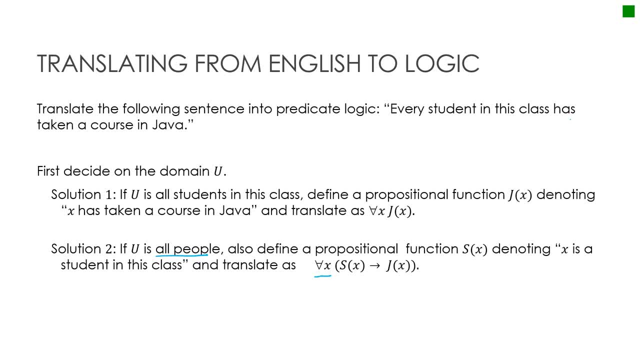 let's a look at how we write that for all X. and then now I'm saying if s of X, which means if it is a student in my class, then they have taken a course in Java. so notice the difference between the two, just based on how we really 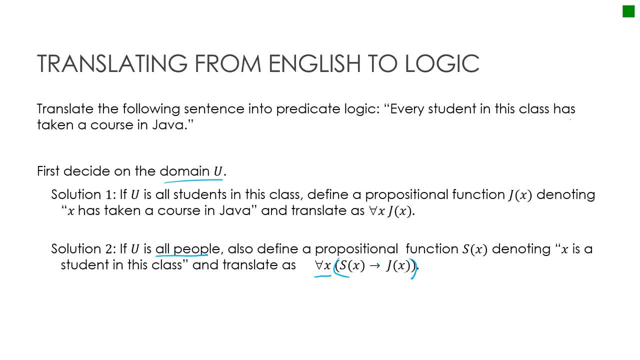 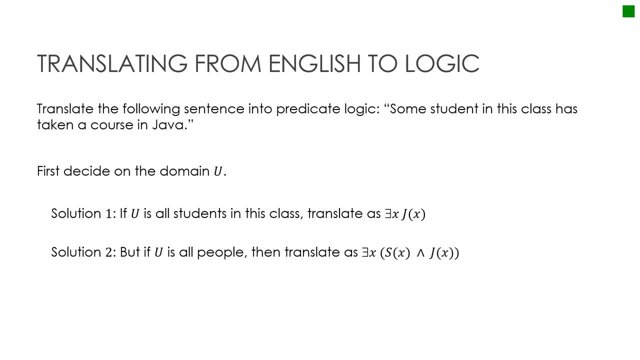 ョی restrict the domain. And another very similar example: some student in the class has taken a course in Java. Again, if U is all students in the class, we already have students in the class taken care of and we're saying some of them. 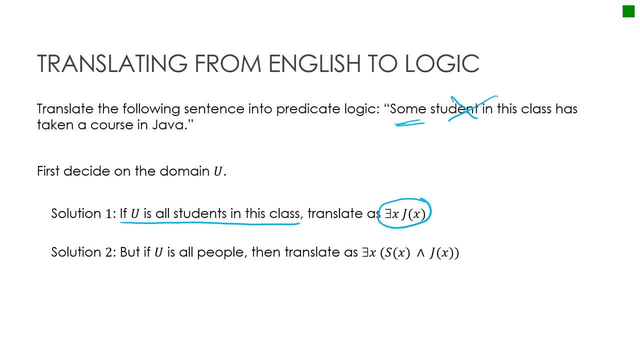 have taken a course in Java, so there exists at least one student who has taken a course in Java. However, if I'm looking at all people, I have to specify: they're in my class and have taken a course in Java, But I'm still using 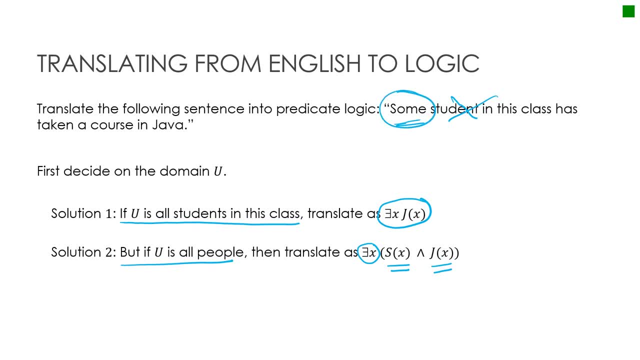 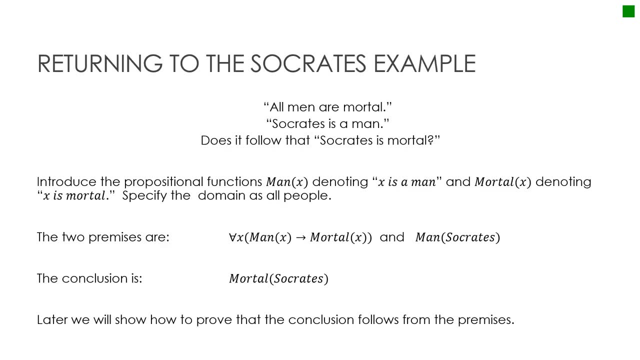 there exists, because I'm saying some. so hopefully this is all sort of coming together for you. So if we look back to our Socrates example from the beginning of the slideshow today we had all men are mortal. The Socrates family had everything they. He's already taken Socrates' family. now she has all of his children, She. 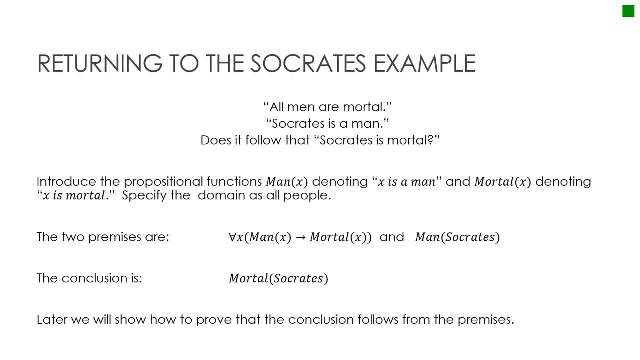 is a man and again, we don't know quite enough yet to be able to come to some conclusion, but we can start getting to that point. we are saying the propositional function man denotes X is a man, the propositional function mortal, X denotes X is immortal and the domain is all people. so we could say the 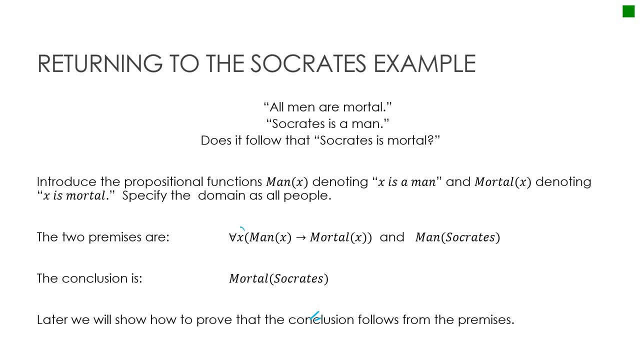 premises as a premises are for all X, so for all people. if it is a man, then he is mortal, and if it is a man or if the man is Socrates, then it's a man. essentially, Socrates is a man. if it is Socrates, then it is a man. sorry, I think I did that one. 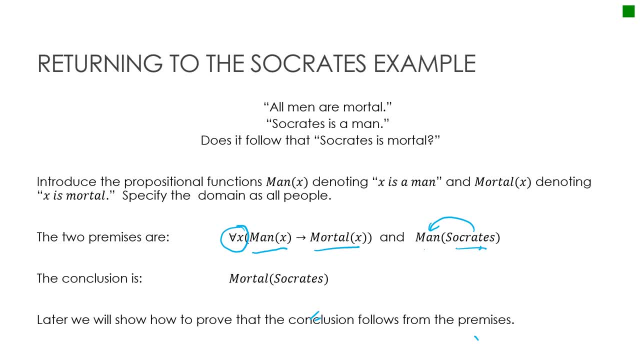 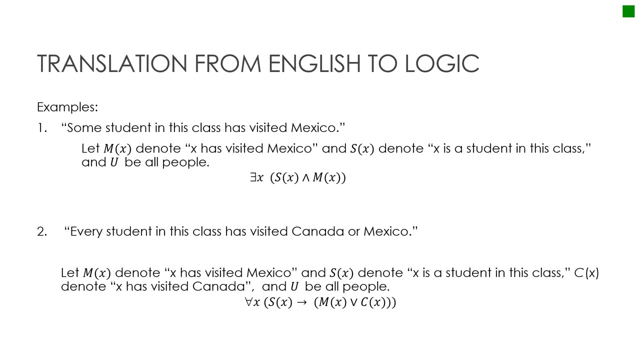 backwards at first. now my conclusion- and again, we're gonna find out how to do that later- but our conclusion would be: if it's Socrates, then he's mortal. but we will get to that later on. let's do a couple more practice together and then I have some for you to try on your own. so 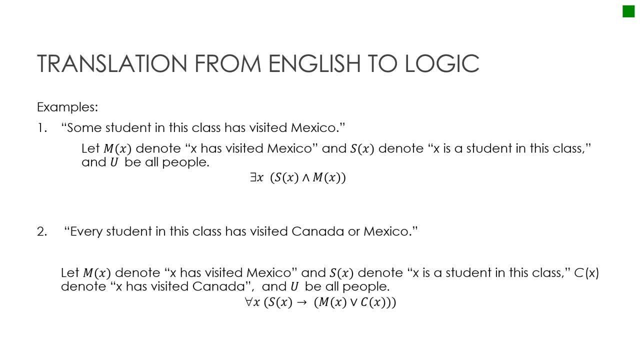 some student in this class has visited Mexico- so remember, here we're looking at some right away that should tell us we're using there exists, as opposed to for all so- and has visited Mexico, whereas this one says every student, so now, right away, you should be thinking we're using for all X. every single student in the class has. 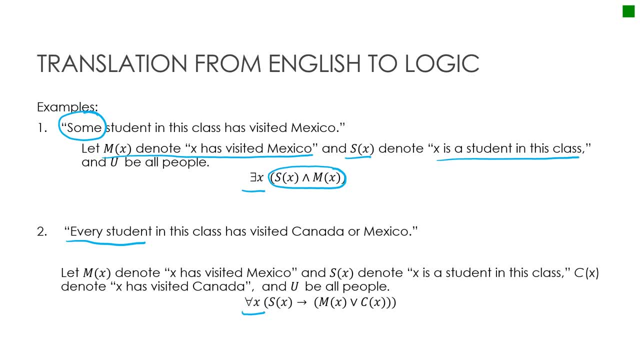 visited Canada or Mexico, again this one also through Canada in there. so now we're using C of X for Canada, so this one is a. if the student is in the class, then they have visited Mexico, Mexico or Canada. and again for allx, every student. and then s of X saying 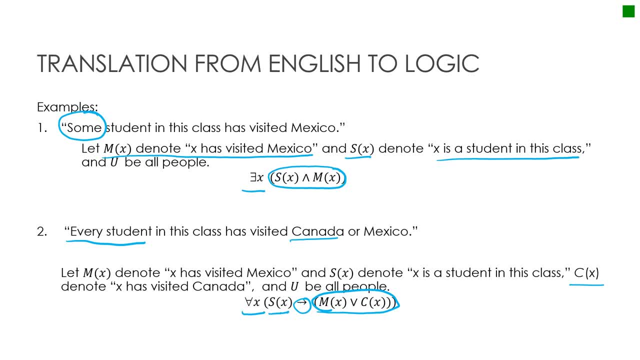 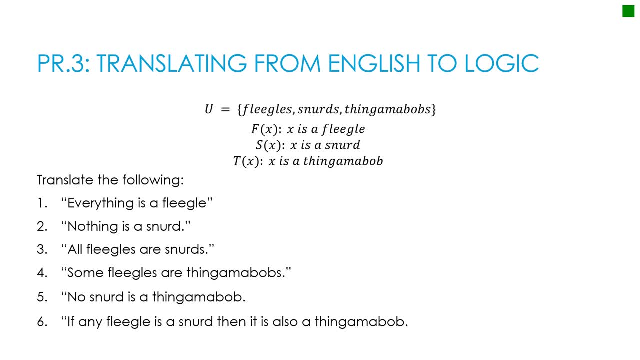 they're a student in the class and if they're a student in the class and then they visited both Mexico and Canada. okay, here's a little fun for you using Flegals, Snurds and Thingamabobs. I would like for you to translate each of the following using f of: X is a Flegal and en Lucas is an. English reading out for it. so let's find out what they said. and they guts. Example: doing everything to Cory was a mess. you're not tired? see, we got good stuff. but at this point I'll be looking at the smartest question ever. I figured we're gonna. 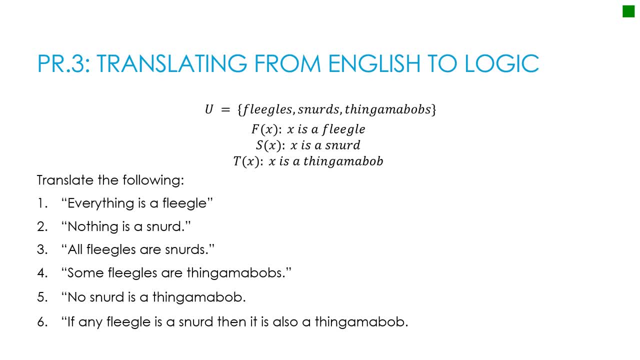 I'm not allowed to do this, but I would t settle for Nothing but a ban, which is because I can't Flegal. S of X is a snared and T of X represents T is a thingamabob. So press pause, take a few minutes to do all six and then press play to see how you did. 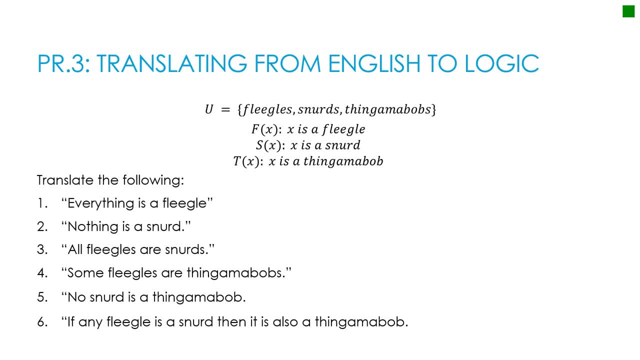 So first one: everything is a Flegal. So hopefully we know that means for all, for all: X, F of X, F of X being X is a Flegal. Well, nothing is a snared, nothing which means either. one of these would be just fine.